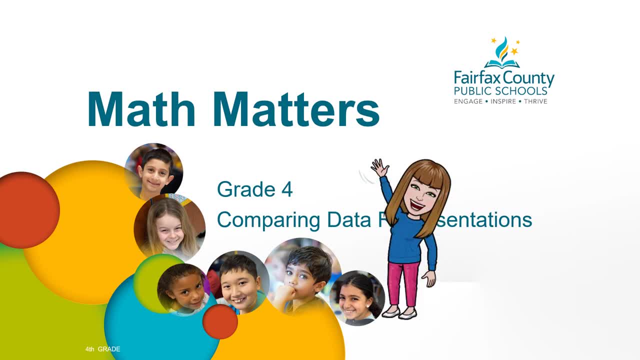 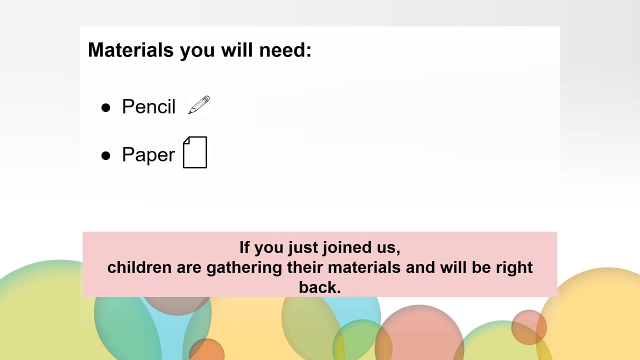 Hello and welcome to this fourth grade episode of Math Matters. I'm Ms Ott and today we are going to compare different representations of data For today's lesson. you will need a pencil and paper. Go ahead and get those items while we wait. 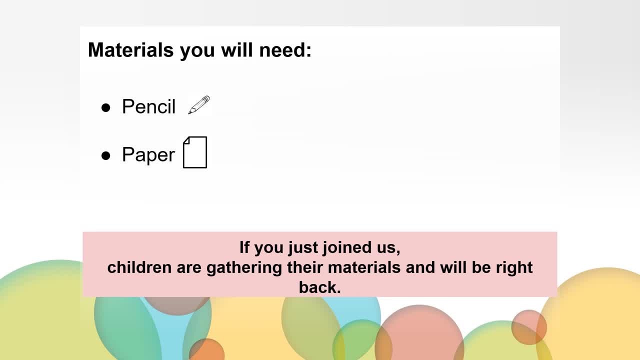 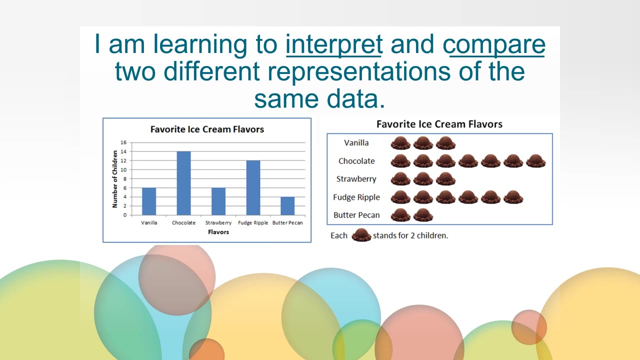 Today you will be learning to interpret and compare two different representations of the same data. On the screen you can see a bar graph and pictograph. Both of these representations show favorite ice cream flavors of some children. But what does it mean to interpret and compare It? 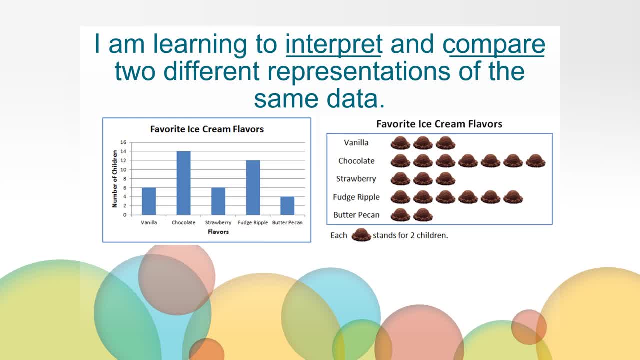 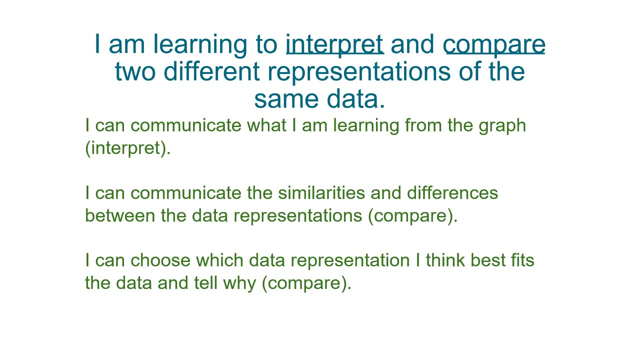 means that we will use the representations to get information and then think about what is the same and different, about the ways we are seeing the data. You will know that you are on your way to meeting the learning goal when you can communicate what you are learning from the graph. communicate the 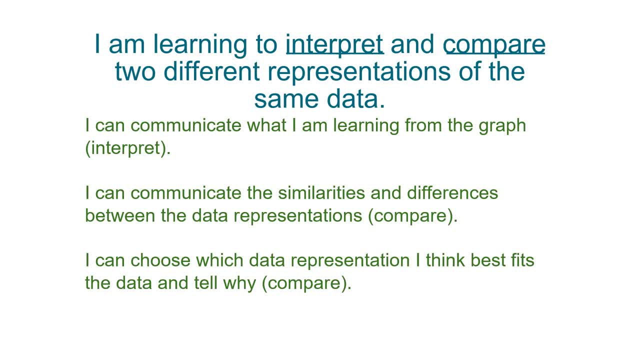 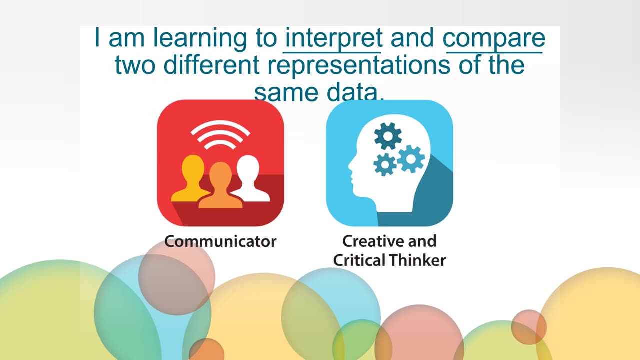 similarities and differences between the data representations and can choose which data representation you think best fits the data and share why. Throughout the lesson today, you will be interpreting and comparing and sharing your thinking either in words or in writing. When you do this, you are a 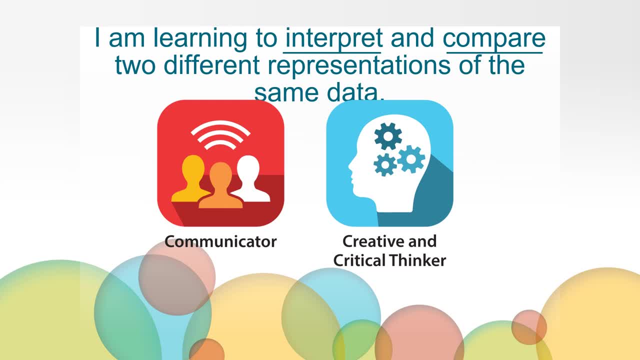 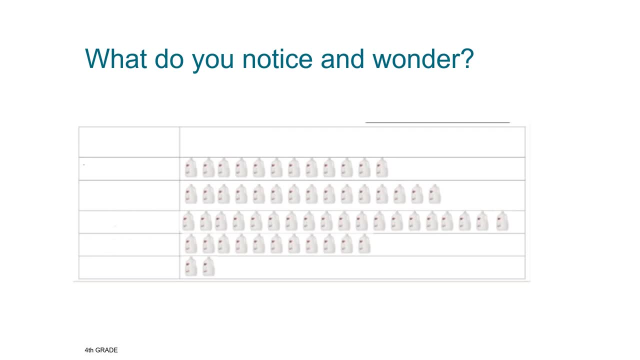 communicator and a creative and critical thinker. This is part of a picto or picture graph. What do you notice about it? Share your thinking out loud. What are some questions you have or what do you wonder about the pictograph? Share your questions out loud. 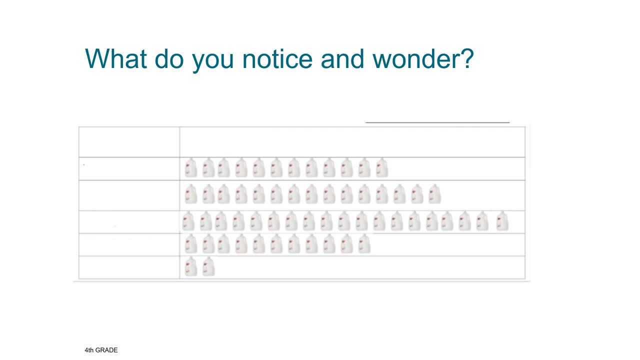 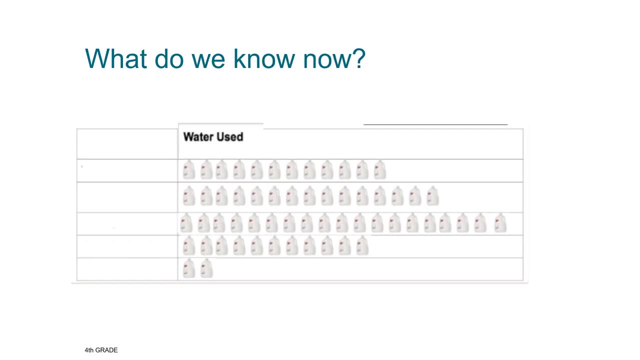 If you have any questions about the pictograph, please ask at the end of this video. Now we have some new information. What do we know now? We now know that this pictograph is showing information about the water used. Now we have more information. What do we know about the water used? Share your thinking. 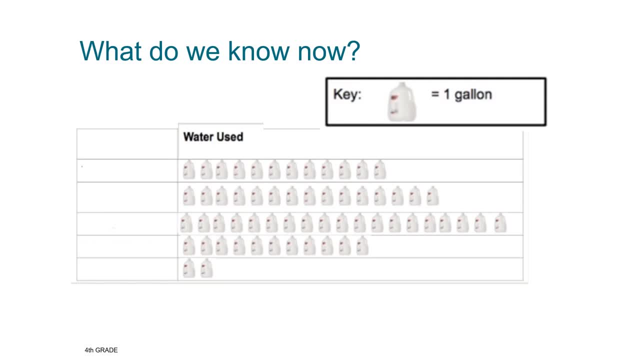 What do we know about the water used? Share your thinking. What do we know now? We now know that each picture in the graph represents one gallon. What do we know now? We can now see that this pictograph is telling us about water uses in our homes, and that one of those water uses is using sink. 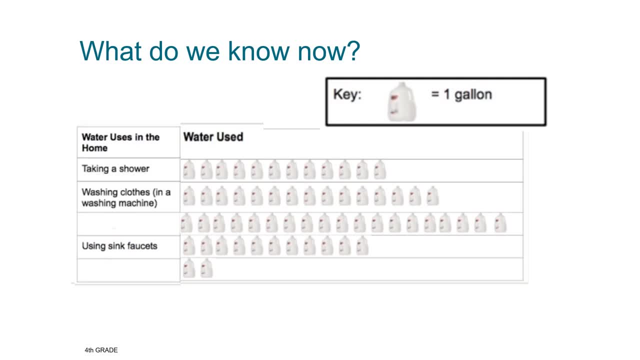 faucets. Now we can see how much water taking a shower and washing clothes in a washing machine uses. Whatever is here uses a lot of water. I wonder what it could be. What do you think? Now we have a picture of a water tank. 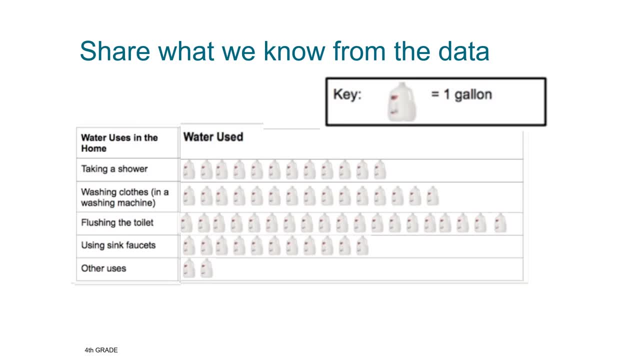 We have all the information needed in our pictograph. Now it's time to interpret the pictograph. Write down three things that you can learn from this pictograph. Maybe you wrote down ideas like flushing the toilet uses 19 gallons of water, or taking a shower uses 12 gallons, Or maybe you noticed that other uses of water in our home only use two gallons. 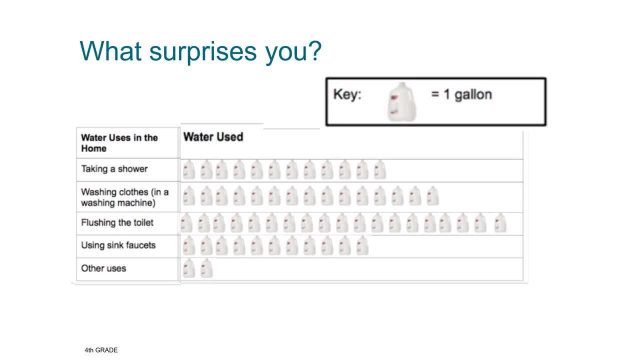 What surprises you today? Let us know in the comments below. What can we tell you about this data or what questions do you have? Maybe you were surprised that flushing the toilet uses more water than taking a shower. Maybe you were surprised that flushing the toilet uses more water than taking a shower. 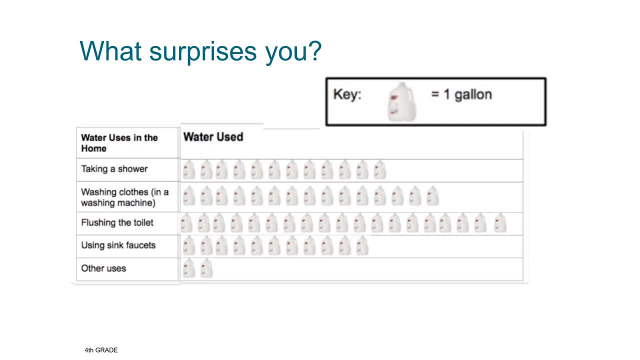 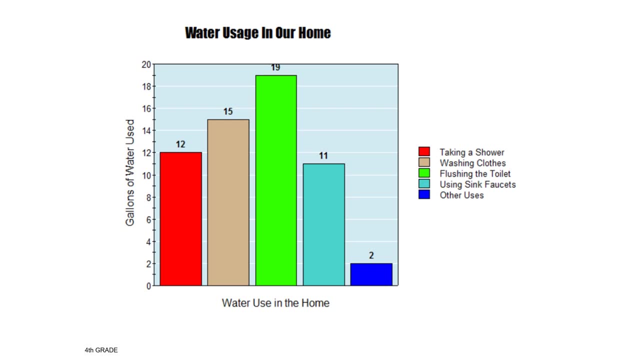 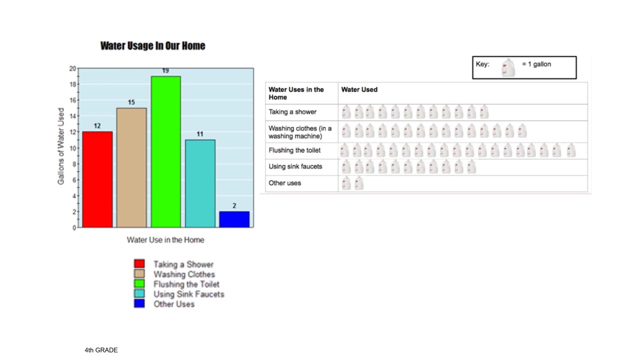 I'm also wondering what other uses of water in our homes is this graph referring to? Let us know in the comments below. Here is the same data about water usage in our home as a bar graph. What are some things that are the same about the two representations. 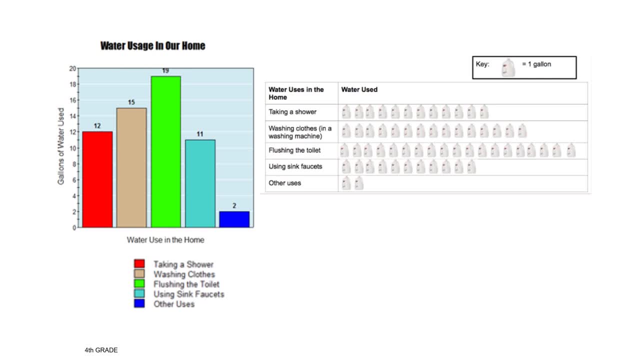 What are some things that are the same about the two representations. Maybe you noticed that both representations tell me what we're measuring in gallons of water. On the bar graph it's listed as the label on the y-axis. On the bar graph it's listed as the label on the y-axis. 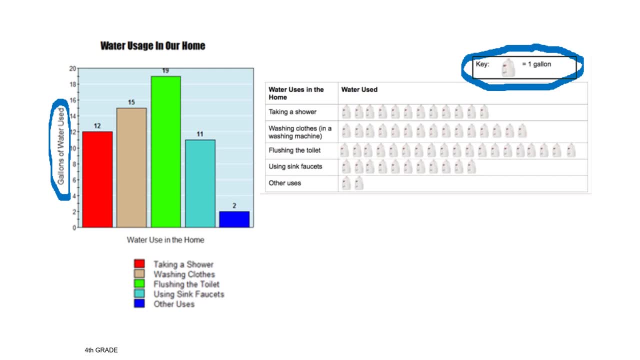 And in the table it's the key. Perhaps you also noticed that the labels are the same. In the bar graph they're listed as a key below the x-axis And in the table they're listed down the left-hand side. 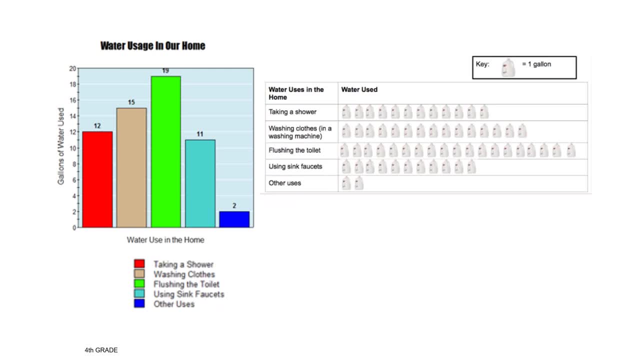 Maybe you also noticed that the number above the bar. Maybe you also noticed that the number above the bar matches the number of gallons listed in the table, For example, for taking a shower. I see 12 gallons in the pictograph and the number 12 is above the bar for taking a shower. 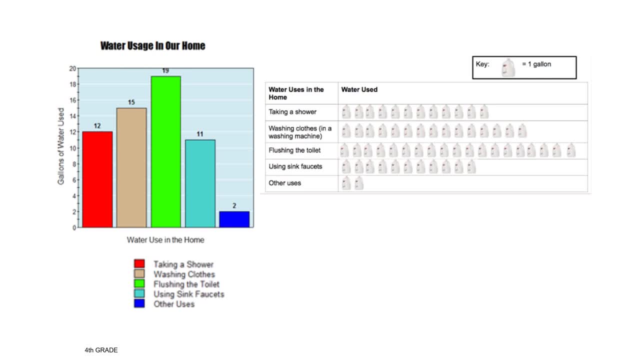 What are some of the differences between the two representations? Share them out loud or write them on your paper. Know the geben prophesy and remember them. say that it's true because you're not sure how, though, although animals do paint, and they know what colors they're, mean to you. 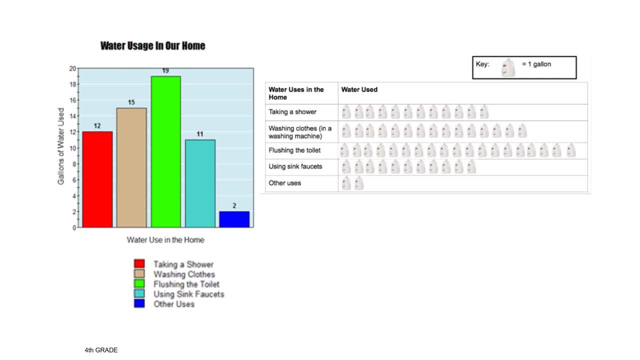 and maybe in the image that you're able to see them again, you see that they're present in the words. it's more visible. One difference is that the bars go up vertically in the bar graph, but in the pictograph the gallons are listed horizontally. 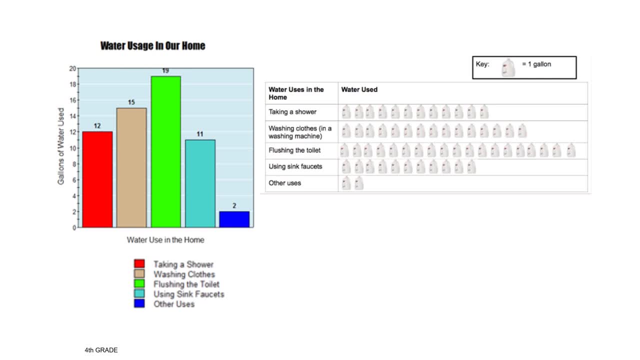 Another difference is that I can see each gallon that it takes in the table, but in the bar graph I can't see each individual gallon. I can only see where the bar stops to tell me the total. What other differences did you notice? 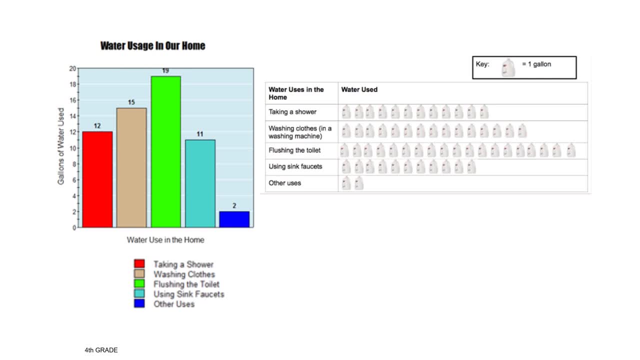 Both representations show the same data. Which one do you prefer? Why do you prefer that one? Communicate your thinking out loud. Now, let's use some critical thinking skills. If you were trying to convince someone to use less water at home, 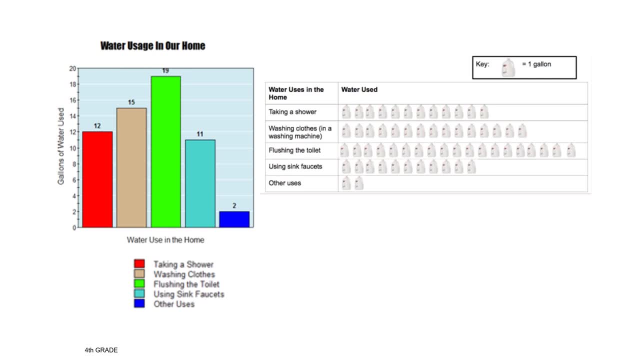 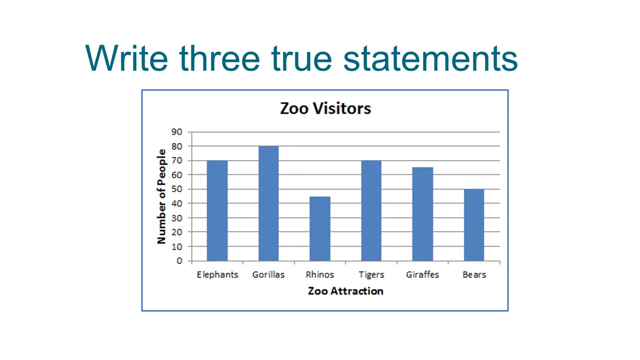 which representation would you show them? Why would you choose that one? Share your thinking out loud. Let's get some information, or interpret a new graph. This bar graph shows the number of zoo visitors to the animal exhibits at the zoo. On your paper, write three true statements. 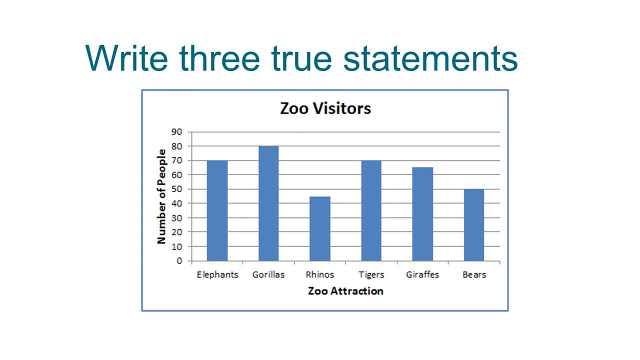 according to this graph, The first one is the number of animals. If you're looking at the number of animals in the graph, which one of the animals is thefinest in the graph? You can see that the first one is the homework. 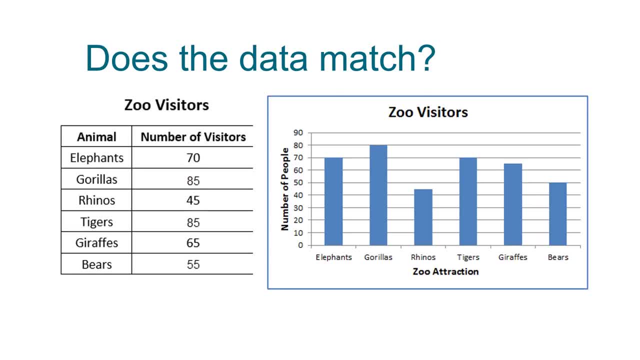 The second one looks very similar to the number of animals in the graph. This is the information about the number of the animals in the graph to the number of animals that go to the zoo. The last one is the number of animals in the graph that was reported to the bag. 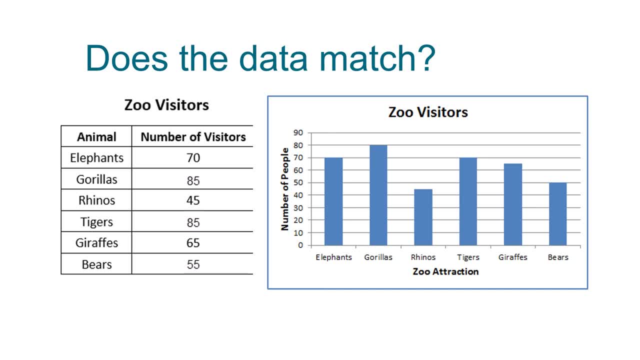 Let's get an idea of the second: the number of dogs that were reported to the zoo. How can you make this data groups that match the data on the bar graph? By comparing the number of visitors in each set, I can see that the data does not match. 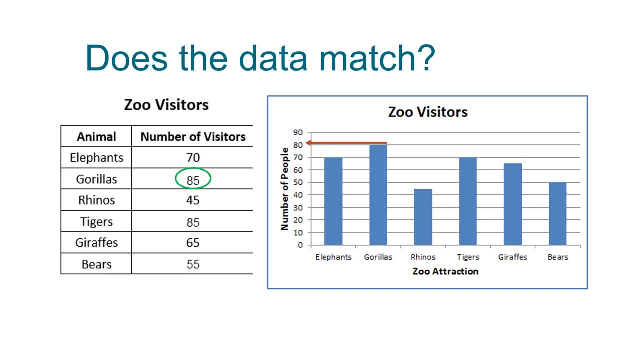 In the table it says that there were 85 visitors to the Gorillas, but according to the bar graph there were 80. So these two data sets do not match. Does the data in this table match the data in the bar graph? 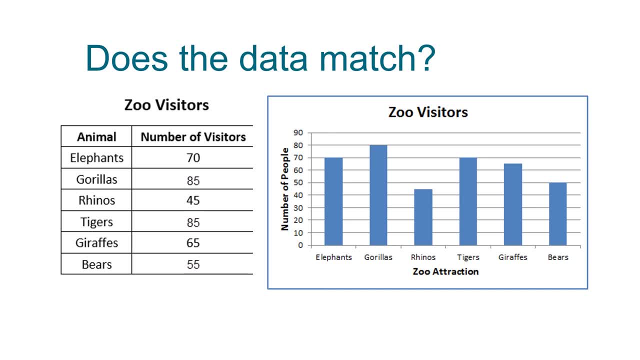 These data sets do not match either. I can see that in the table there are 85 visitors to the Tigers, but according to the bar graph there were only 70, and that in the table it says that 55 people visited. 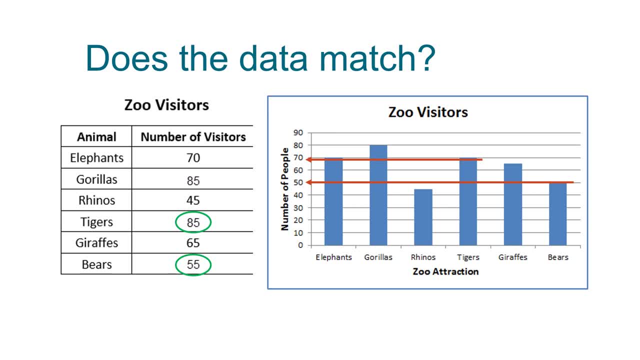 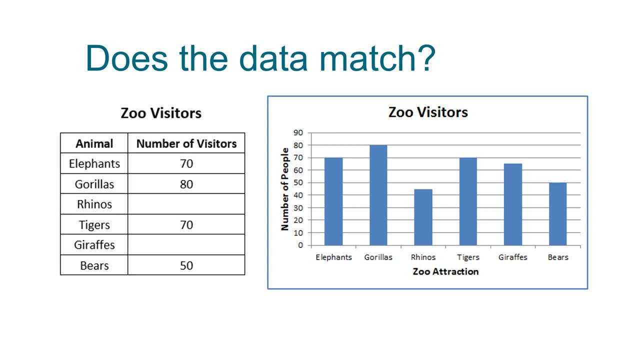 the Bears, but on the bar graph I can see that 50 visited the Bears. These two data sets do not match. Here is a table with some missing information. With the information that we have, does the data in this table match the data in the bar? 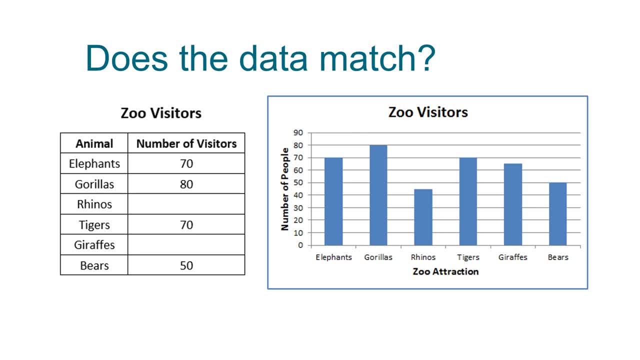 graph. So far, the data is a match. What numbers would we have to add to the table so that it continues to match the data in the bar graph? Write the two numbers down on your paper. The bar graph tells us that there were 45 visitors to the Rhinos and 65 visitors to